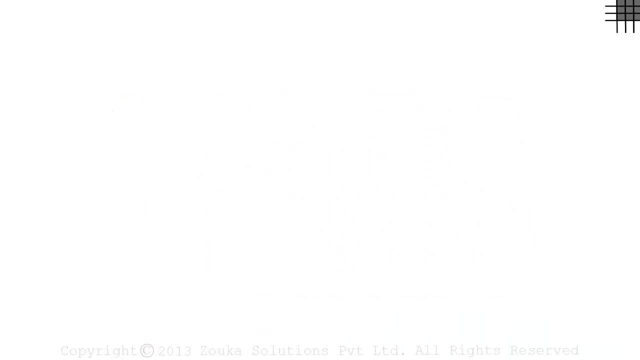 The concept of proportion is very simple. All we need to do is understand a couple of simple examples. Assume you have a computer screen of the size 40 cm by 30 cm at home And you've been asked to draw that screen in your notebook. 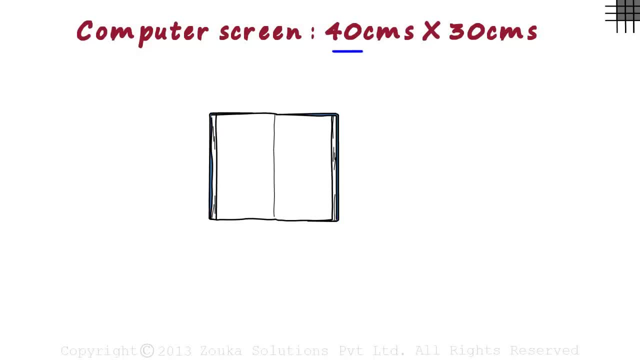 What do you do then? You cannot draw a 40 cm by 30 cm screen in your notebook. Your notebook would be too small for that. So what you do is scale the size down. This term is very important. You scale the size down. 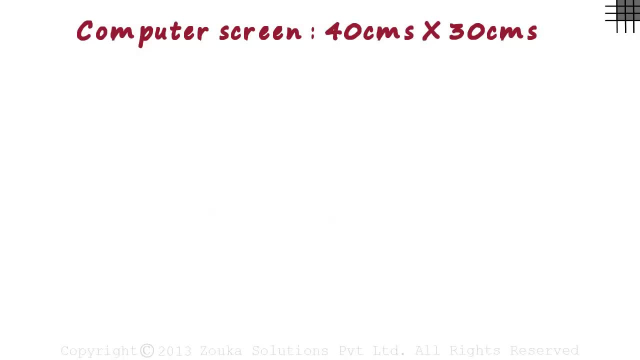 It means you draw a smaller figure which is similar to the earlier one. You may draw a small screen like this With length 4 cm and width 3 cm. This will fit into your notebook. Here the ratio of the length to the breadth: 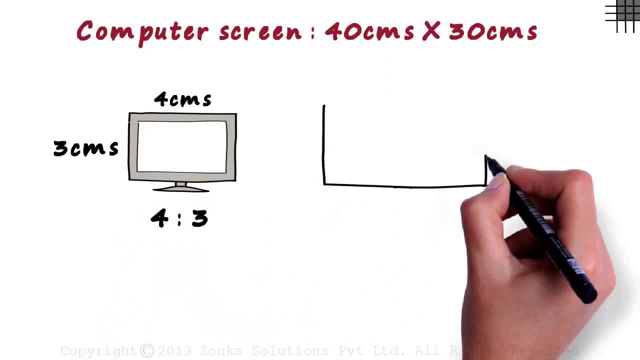 is 4 is to 3.. If you had a bigger book, you would have maybe scaled it down to 8 cm by 6 cm. In this case, the ratio of the length to the breadth would be 8 is to 6.. 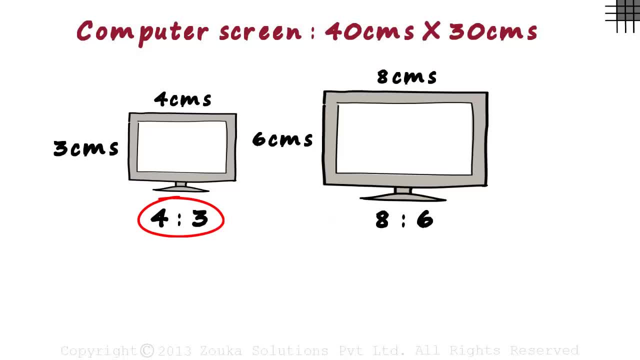 Let's talk about the first case. Why 4 is to 3? The ratio of the length to the breadth of the actual computer screen is 40 by 30. When reduced it can be written as 4 by 3.. Basically, if we divide both the numerator and the denominator by 10,. 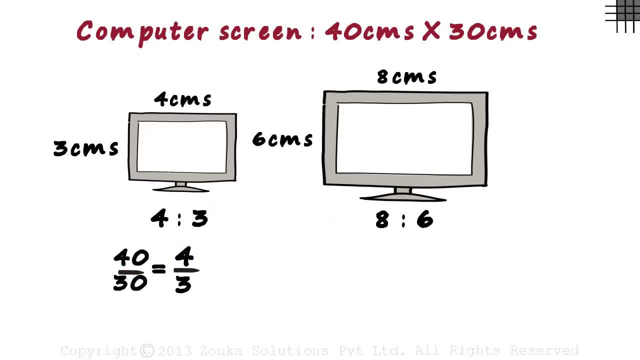 we get 4 by 3.. Now let's look at the second case of 8 by 6.. The ratio of the actual screen was 40 by 30. If both the numerator and the denominator are divided by 5, we get an equivalent ratio of 8 by 6.. 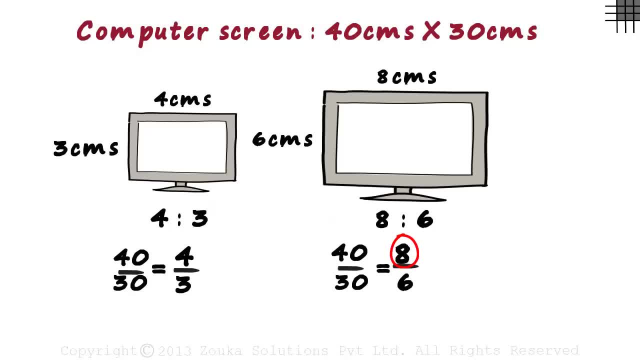 40 divided by 5 equals 8, and 30 divided by 5 equals 6.. What did you notice in this example? What are we trying to maintain? We are trying to maintain the same ratio, All the three ratios: 40 by 30,. 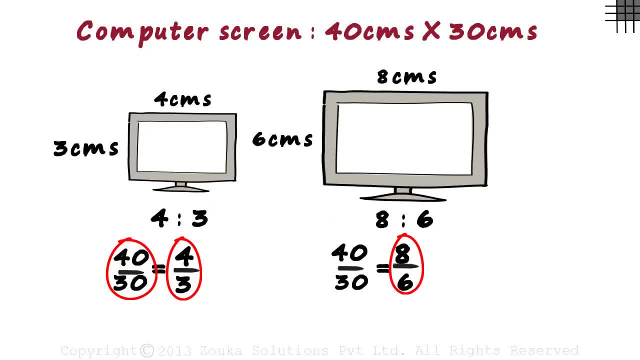 4 by 3 and 8 by 6 are actually equal. We just changed the numerator and the denominator based on the requirement. Here we had to draw a smaller screen, and hence we reduced the numerator and the denominator proportionally. That's proportion.